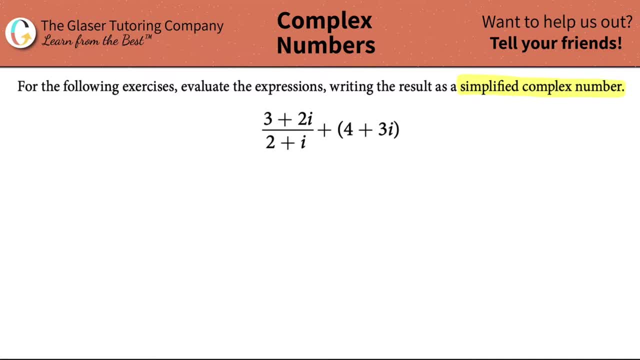 number videos that we've done. you can click on the playlist- The link is in the description- for that, as well as all of our other math playlists, If you want to go back and see what we've done. we've got everything covered for you guys. 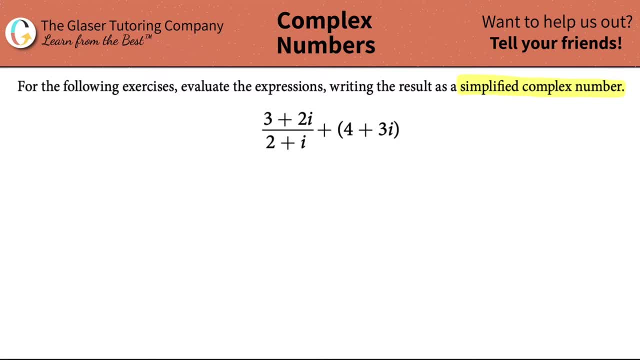 So, without further ado, let's get down to business. We need to simplify this whole mess, right? We need to simplify three plus two, I, divided by two plus I, and then it's all being added to four plus three I. So I'm looking at this from a simplifying standpoint and I want 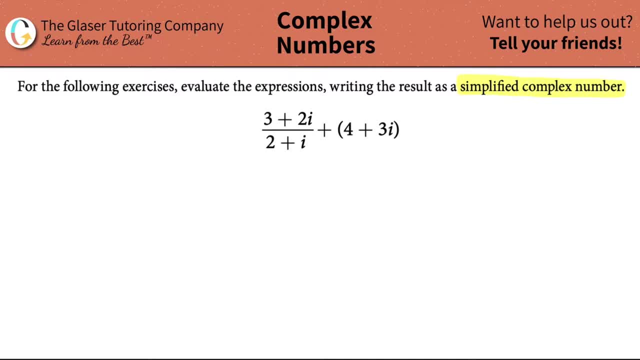 to see what am I going to do. first right: I know, according to PEMDAS, that multiplication and division, so dividing comes first before I add this stuff out. So I know that I have to work with this first right And I know from all the questions that we've done that the problem arises. 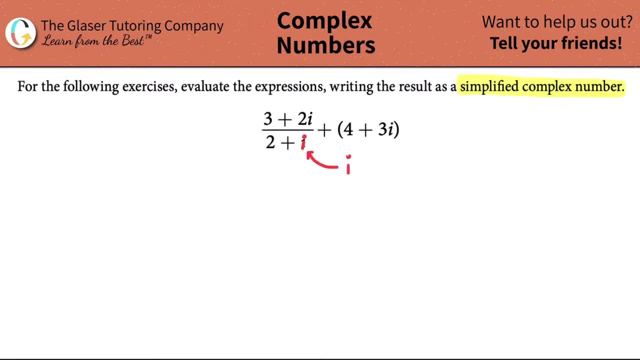 here, In which your- I value, your imaginary component can never be in the denominator. So I know that I'm probably going to have to start somewhere by working on this denominator and trying to get rid of I in that denominator. So how are we going to do that? Well, we know that we will. 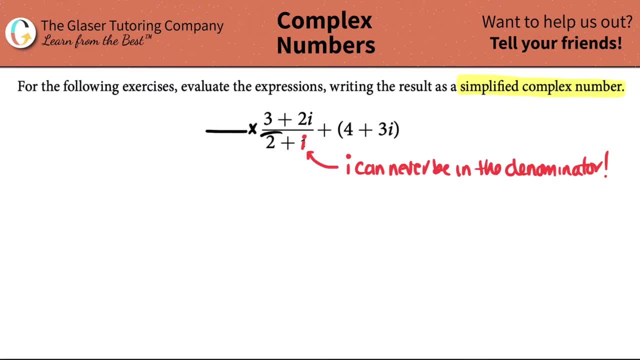 always just multiply by the opposite of I, So we're going to have to multiply by the opposite of what's being done here. So if I'm doing two plus I, I need to multiply by two minus I in order to get rid of that. I value, But I got to be fair If I multiply the denominator by that number. 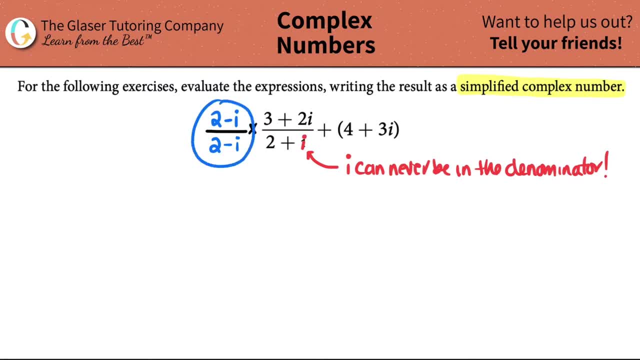 I have to multiply the numerator as well, And this is why we can multiply things randomly at thin air, because this would just simplify to one And really in retrospect we're just multiplying by one, but we can actually do the math to get rid. 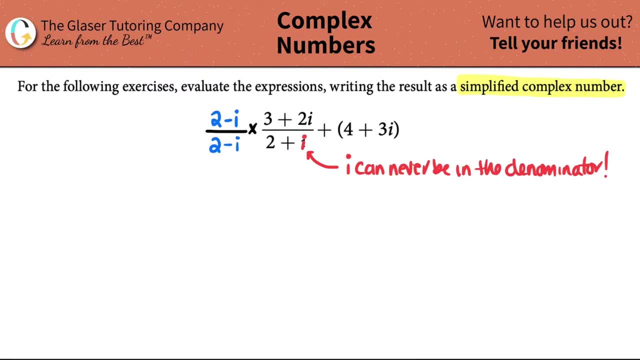 of the I value. So it looks like I have now two things that I have to multiply. I need to multiply the top right by this, And I need to multiply the denominator as well. It doesn't matter which one you do first, You just got to do one and then do the other. Let's work on the denominator first. 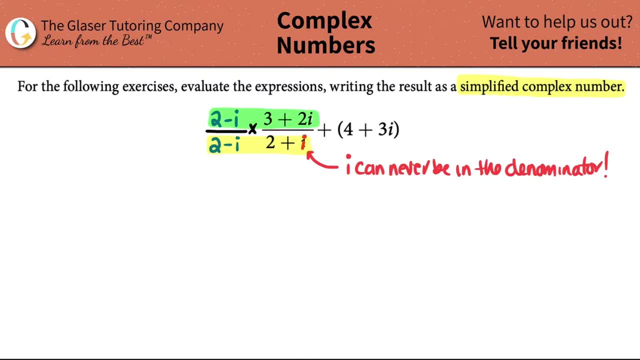 because that was the whole idea why we had to do this mess: Because we want to get rid of the denominator, the I and the denominator. So essentially you have these two parentheses being multiplied by each other. So I have two minus I, And you know. 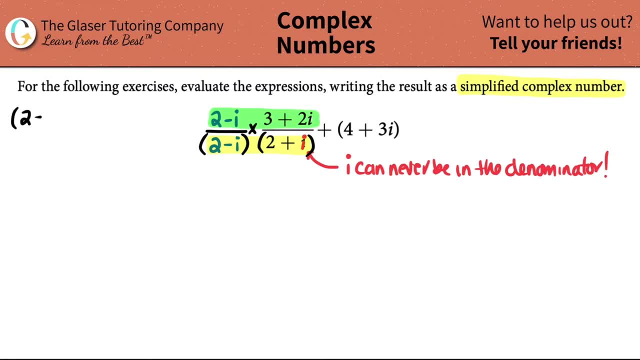 what? Let me start up here because I'm probably going to need a lot of room. There's been a lot of work being done for the past couple of questions. These are hardcore. So two plus I. Okay, So I have two minus I times two plus I, And we've seen this idea. 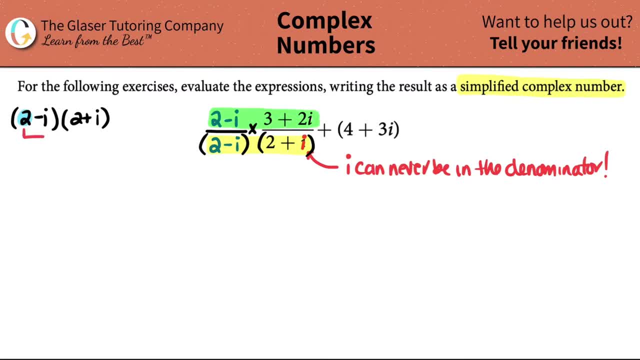 Tons of times. right, The two has to be multiplied by that first guy. And then he wants to be multiplied by the second term. But then you got to be fair. If you're going to multiply the two, you got to multiply by the negative I by the two and the I. So there's four multiplying steps that 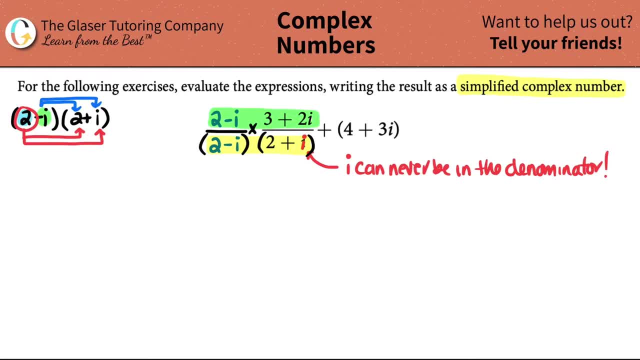 you have to do. Let's get started. Two times two is four. Two times I is a positive two I, So plus two I. Then, if I'm moving on to the blues, negative I times two is negative two I, And then 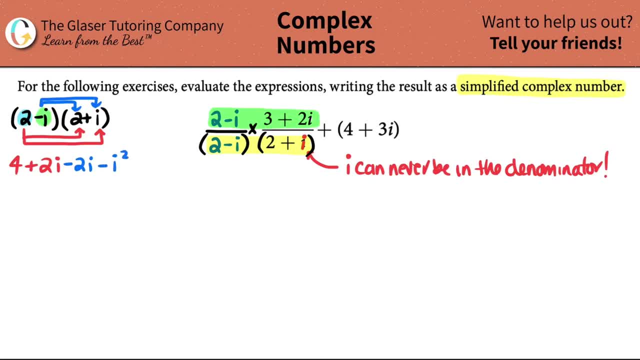 negative I times. I is a negative. I squared. You had two I's, So you represent that by a two. Okay, Clean this up, right. I have two variables with the I value in it. Two minus two, right, And I'm taking it from here: Two minus two is. 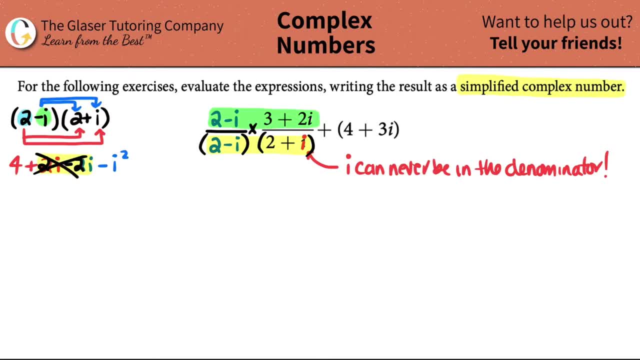 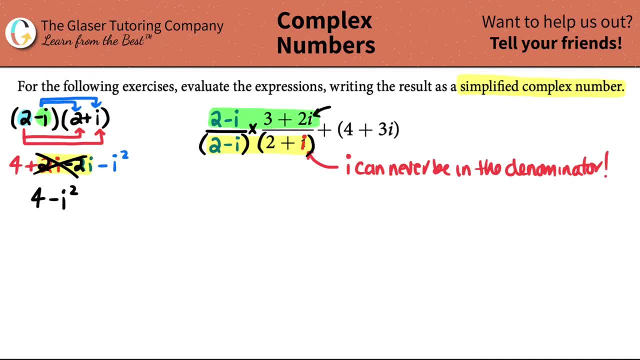 in my answer. right, I can't have I squared or I cubed, or I to the fourth, So I need to get rid of this. But we can get to that answer by saying: well, what does I really mean? I is the square root of negative one. It's a square root of a negative number, right, If we? 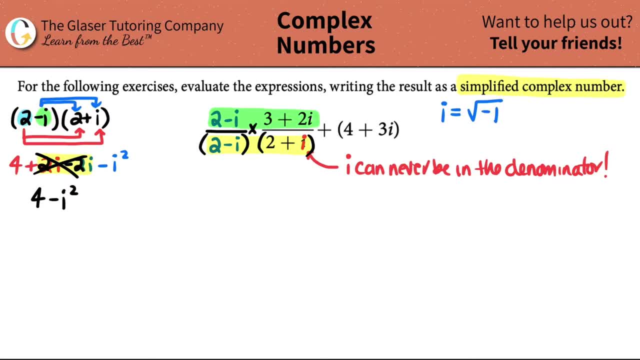 plug in a square root in our calculator of a negative value, the calculator is going to decompust and break up. Maybe not, but it'll. it'll just give you an error. right, If you put in a square root of negative 25, the calculator is going to say error because it's imaginary. 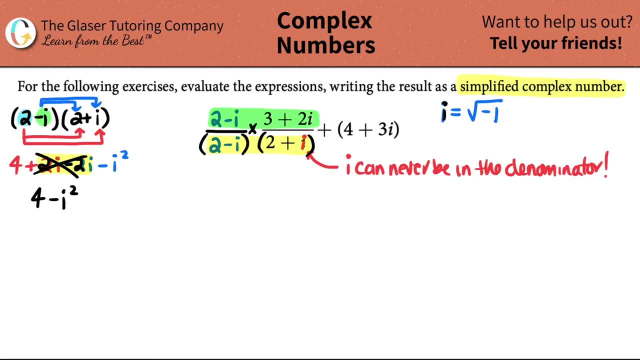 It's not real. It has I values to it. It's an imaginary world. So if we're going to solve for an I squared, that means that I just have this, the I value which is this squared. So this is just saying that I have a square root of negative one squared. And what is? 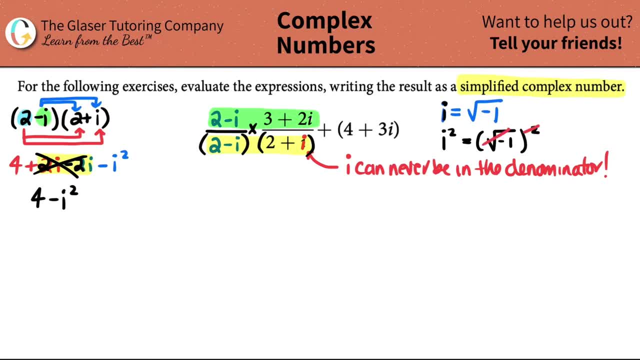 a square root being squared. They're opposites of each other, So they get canceled. So that's your answer. An I squared always equals negative one. So that's what's going on here. So this really equals just a negative one. So this would be four minus. 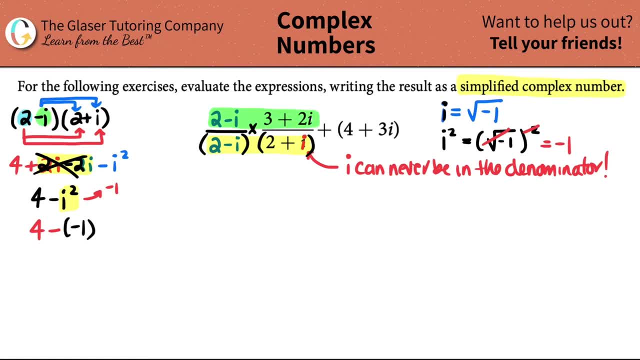 a negative one, four minus a negative one. Keep change, change. This is just a five, So that means that the answer. actually, I don't want to say that, I will just say that this whole thing- if I break this down right, Because that's what we're doing- 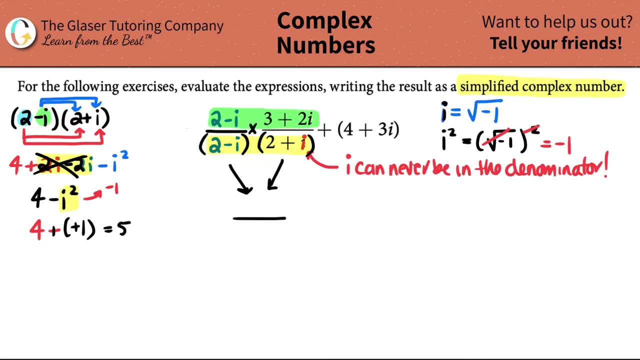 This multiplied by this, the denominator for the whole thing is the square root of negative one squared. So this is just a negative one squared. This is five. right Now we have to do the work, to do the numerator, And can you guys see that? 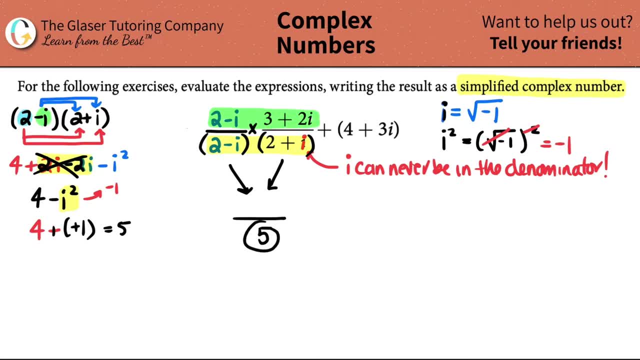 there's. there was I's here, Now there's no more I's, And that was the problem. So we fix the problem. Now we just have to do the numerator, So that's two minus I times three plus two I, And the same exact idea is happening here. 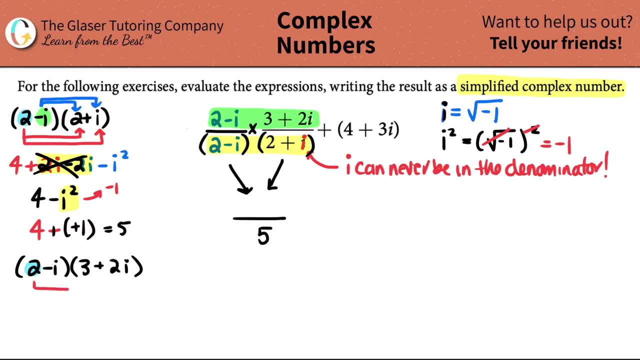 So I have to multiply the two by the three and the two I. And then I have to multiply the negative I by the three and the two I. So four steps again. Let's give it a shot. Two times three is six. Two times a two I is a plus four I. 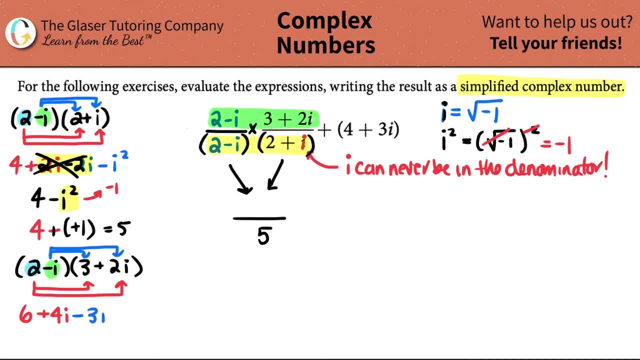 Negative I times three is a negative three: I Negative I times two: I is a negative. two: I squared. Let's clean this up: Four: I minus three. Four minus three is just one, So this would work out to being six plus. you could say one: I, or you can just say I minus two, I squared. 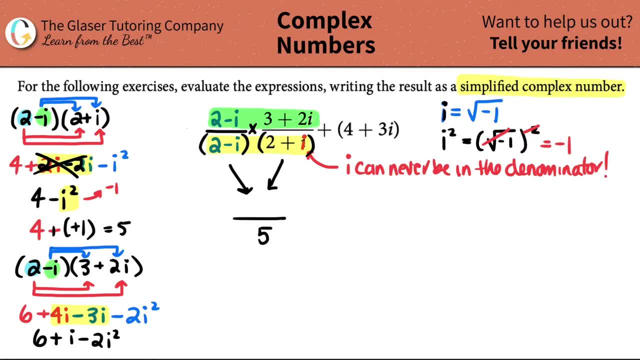 Okay. Well, we run into the same problem as last time. I can't have any, I squareds, but we now know that I squared just equals a negative one. So this would be equal to six plus I minus two times a negative one. 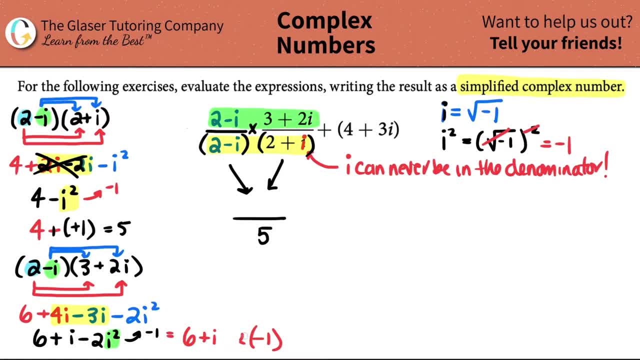 Negative two times. a negative one is a positive two. So I can just erase this and say this is plus two Six plus two is eight. And then I can just erase this and say this is plus two: Eight, And then we just have that I at the end. So that's the ending for this. This is now the 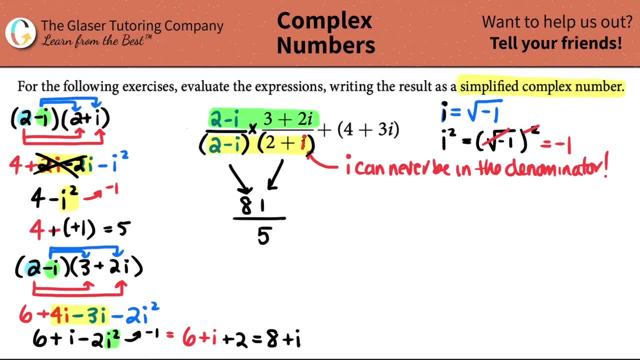 new numerator. So this would be eight plus I. So this whole thing simplified down to one single fraction: eight plus I over five. Now we like to get this even more broken down into real and imaginary components. Remember, if you have multiple things in the numerator, divided by just one single denominator. 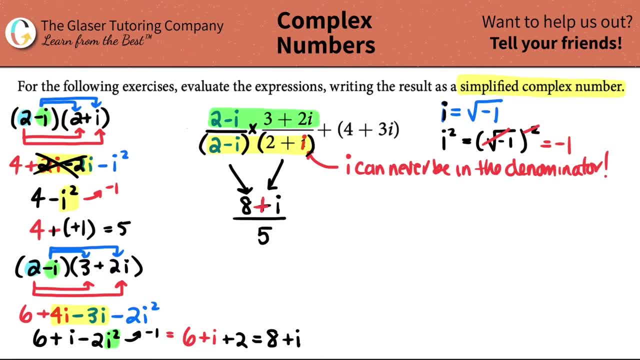 you can break them into parts by their addition or subtraction signs. So this would technically be eight over five, So eight divided by five plus the I over five. And now I have that nice and simple. I have a real component here, I have an imaginary component here. This would be the same thing as saying: 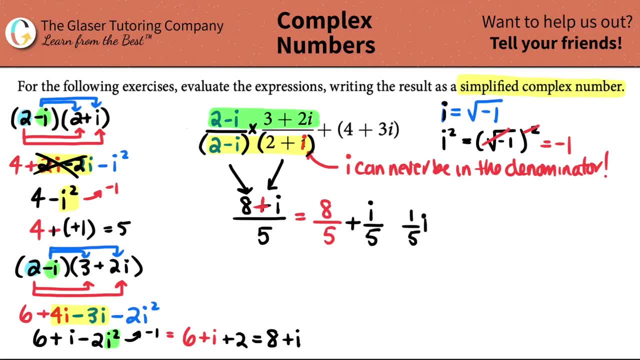 you know, one over five times I. It does not matter. I'll probably use the other one, though, because we still have to plus this whole jazz, So let's just put this into context. Okay, So this is the answer that we just found. However, we're not done. We just did this part, But now we have. 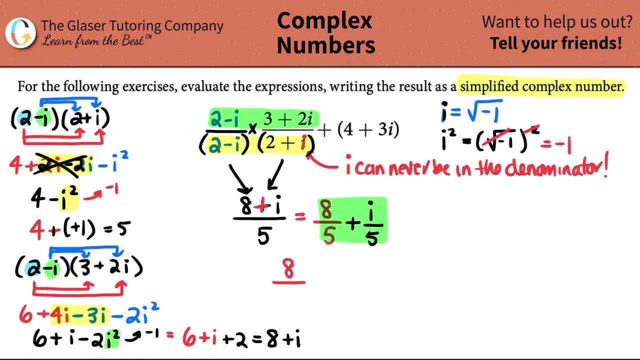 to do If the particular function of eight over five is our Aussie嗎, so 8 over 5 plus i over 5 оus. parentheses. I put the parentheses there because there was parentheses here. However, when you're just adding, you don't need. 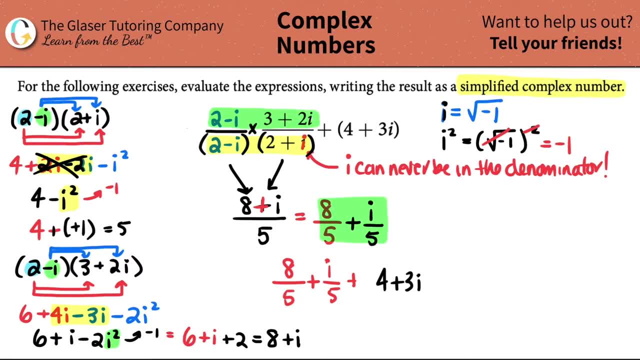 parentheses Right, Because you're not multiplying, So you don't have to play fair. they just put those parentheses there to probably trick you. But now we have like terms, right, I have an eight over five. That's a real component, And I'm going to add that with the 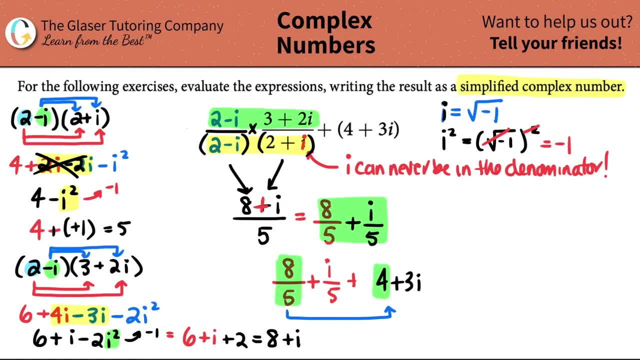 real component on the other side, which is a four, And then I'm going to add together the imaginary components. I have an I over here and I need to add that with an I over here. Notice how I'm saying adding and I'm not multiplying, I'm not playing fair. I don't have to take this eight. 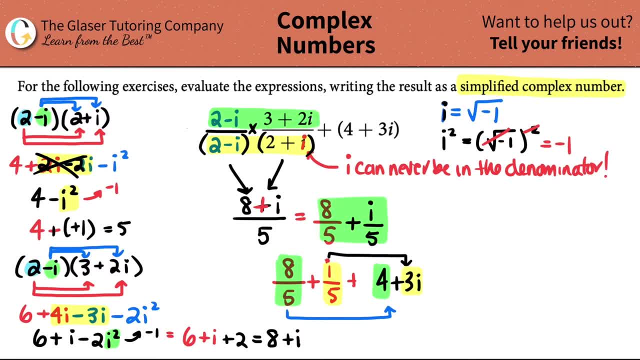 over five and do it to both of them. I can't, because adding and subtracting- you can only add and subtract like terms. So let's take this in two steps. I have an eight over five and I need to add four. Now there's so many ways to do this right. You can use this. You could plug this into: 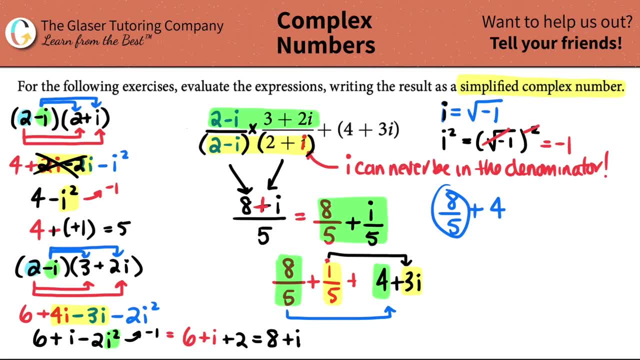 the calculator. Um, you can make this a fraction, um, a decimal, and then put it into the calculator. It doesn't matter to me. I like to work with fractions. I'm probably the only one that likes to work with fractions, So I will work. 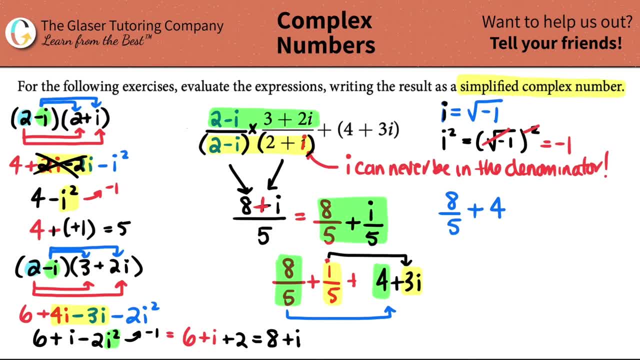 with fractions? Uh, we need to find a common denominator, right? So, basically, what is the same thing as saying four but having a denominator of five? this was technically four over one, right? So if I multiply by five to get the five denominator, I got to be fair, I got to multiply. 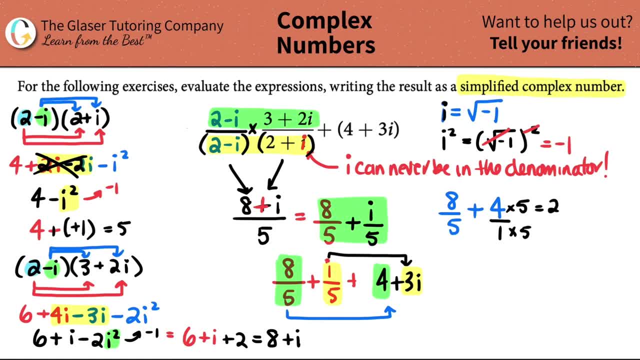 by that five on the top. So this would be the same thing as saying 20 over five. and keep in mind, right, It was a plus four. 20 divided by five is a four. So I can just simplify and say okay. 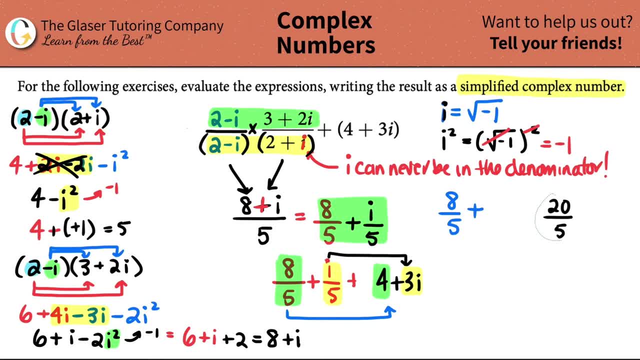 I'm not adding four, I'm adding 20 over five, And now we have a nice little fraction, right? When you're adding fractions, remember you just keep the denominator the same. So just be a five, and then eight plus 20 is 28.. So this is the answer. 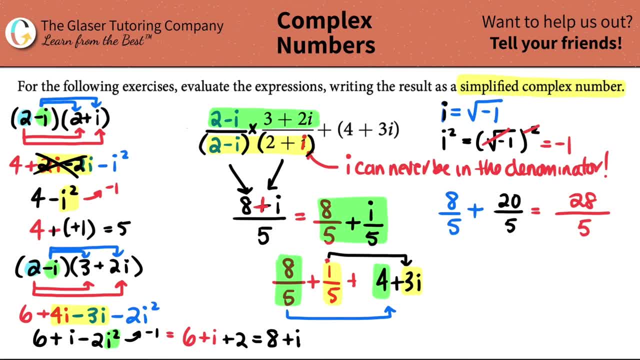 to the first component. Now we're going to do the same exact idea, but with the I values. I have: I over five plus- oh, that was an ugly, that was an ugly. five. I over five plus three, I, Okay. Well, same exact idea. I want to get my common denominator. So remember this was. 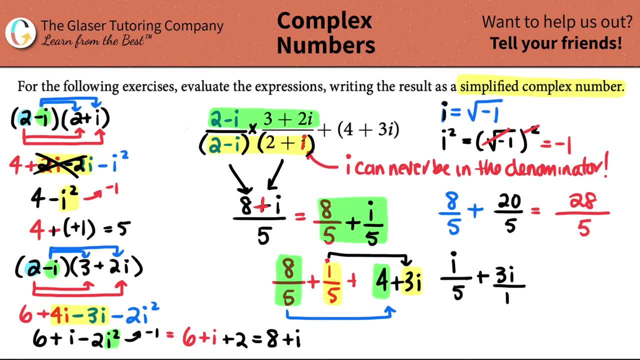 over one and I want to get it into a five. So I have to multiply by five on the bottom. but I got to be fair, I got to multiply it by five on the top, So this would be the same thing as five, and then three times five is 15.. So this is 15, I and remember it just equals three. 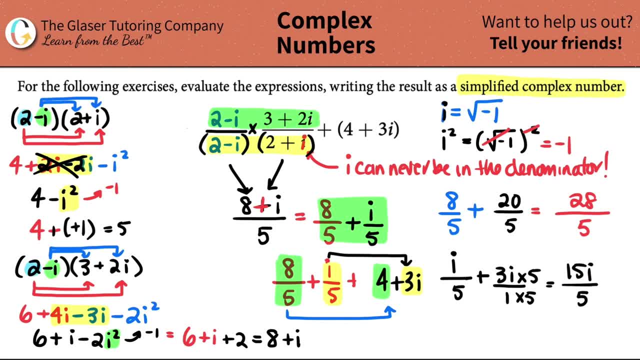 I. but if I simplify this it turns into three I right. So instead of adding three I, I will just add 15 I over five. And there's remember, there's one I here, right. So common denominator doesn't go anywhere. 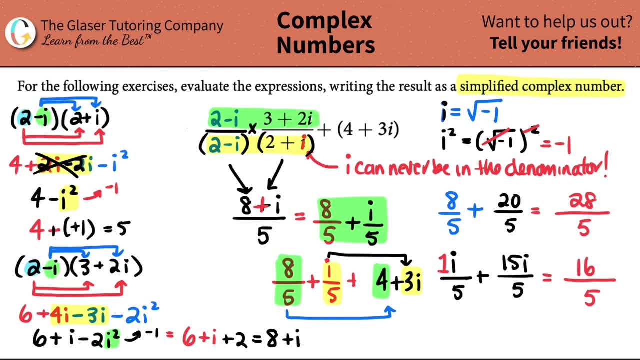 You're just adding the one plus the 15, which is 16.. I and there you go. So it's these two components, your real and your imaginary. they're being added together. So your answer would be 28 over five plus 16, plus 16: I over five. 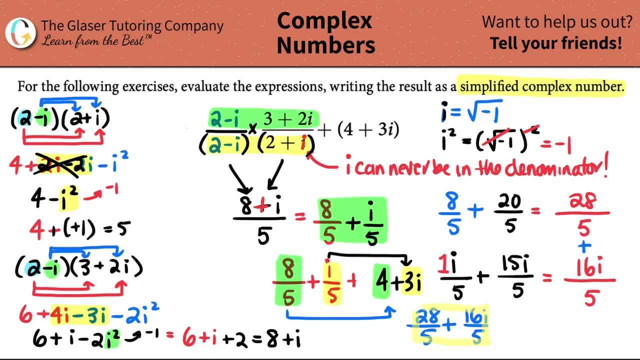 And that's simplified, complex notation. The real value has to come first, The imaginary comes second. But other than that, that's it. And look, I left some space here for the the subscribe button. So if you want to subscribe to the channel and tell us that we're doing a good,